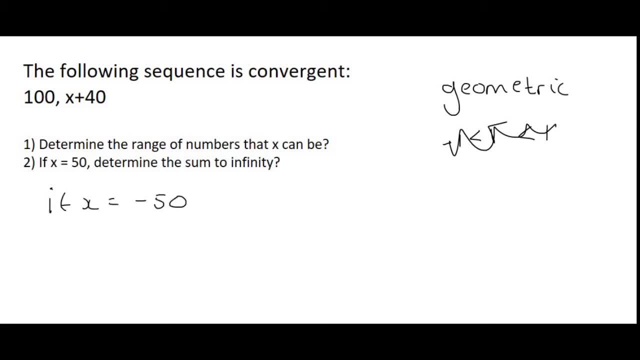 that x was minus 50. Well then, you would have 100 as your first term. Your second term would be minus 50 plus 40, which would be minus 10.. Now how do you get from 100 to 10?? Well, don't worry about the. 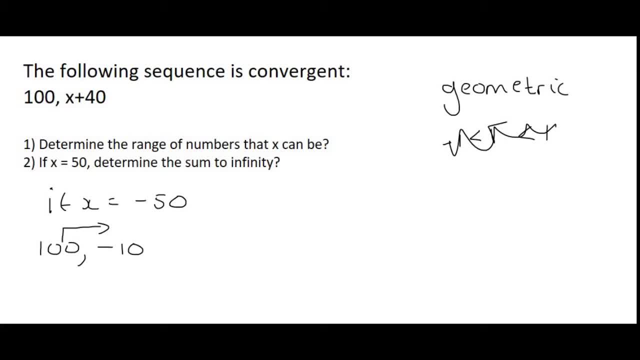 minus. Just to get to 10, you would have to divide by 10. Which is the same as multiplying by 1 over 10.. How did I get that? I said 10 divided by 100.. Okay, but because of the negative, it means our ratio is going to be negative, 1 over 10.. 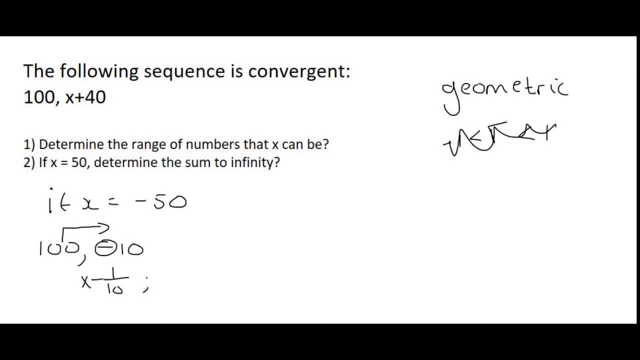 So to get to term 3 you would have to take minus 10 and times it with negative 1 over 10, and that would give us 1.. Then you would multiply that by negative 1 over 10 and that would give us negative. 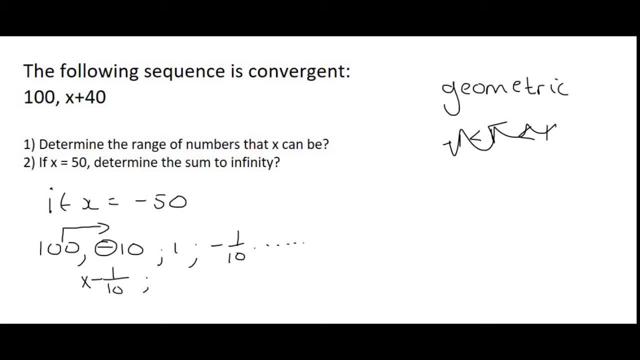 1 over 10.. And as you carry on, you would find that your numbers are getting smaller and smaller. So here your ratio is a negative number, but that is okay. The maths tells us that as long as your ratio is any number between minus 1 and 1, then it will converge. So examples of 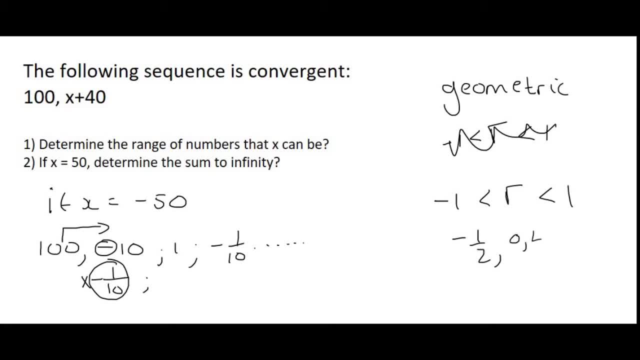 numbers like that would be minus a half, 0,4, for example. Let's do a semicolon there, So 0,4 would work, Negative 0,8.. So we're looking for any number, any ratio number that is between minus 1. 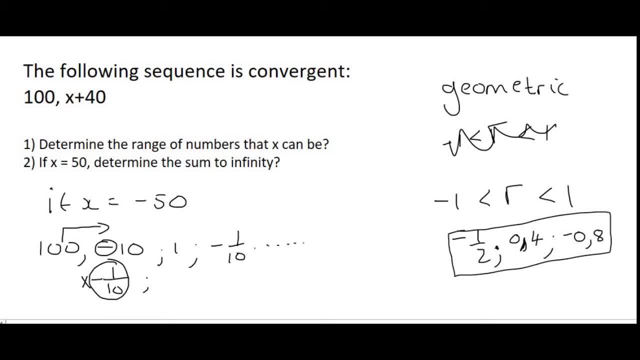 and 1.. So it doesn't matter if it's a negative, as long as it's between 1 and minus 1.. So we found that when x was equal to 30, everything was fine. We said that when x was minus 50, everything was. 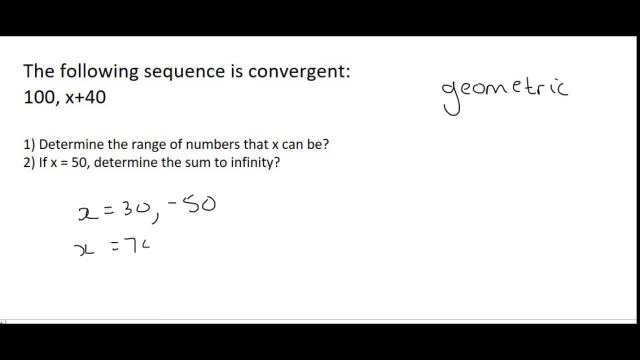 fine When x was 70. then things weren't fine, because then your ratio number became too big. So how are we going to find all of the possible numbers? Well, we want the ratio to be between minus 1 and 1.. How do you work out the ratio? Well, you can do that by multiplying by 10 over 10.. 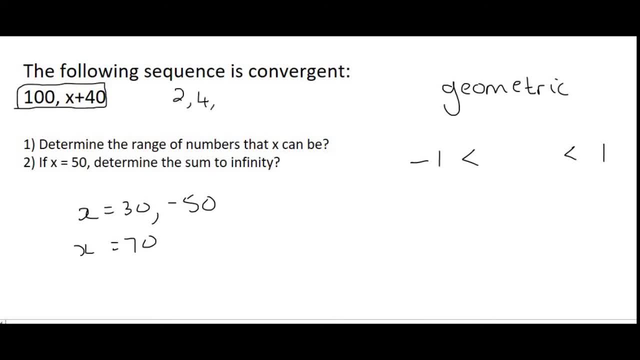 Ratio of this? well, if I gave you a sequence that went 2,, 4,, 8,, 16, your ratio is 2, because it's 4 divided by 2, or you could say 16 divided by 8 or 8 divided by 4.. As long as you choose any number, 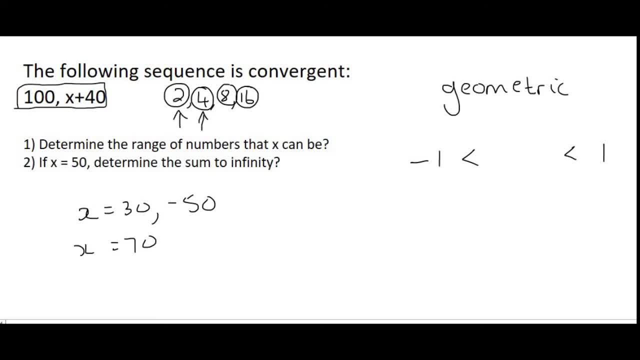 on the right divided by the number to the left of it. That is how you work out the ratio. So in this case it's going to be x plus 40 over 100.. There we go. Now you can just solve that. So we times the. 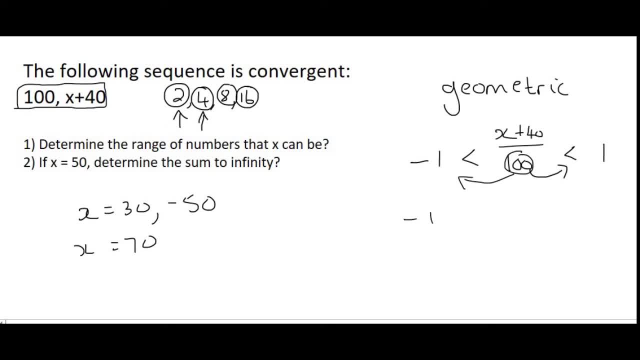 100 on the left, On the right side and on the right side. So we end up with negative 100 smaller than x, plus 40 smaller than 100.. Now if we just move the 40 to the right and to the left, then we're going to end. 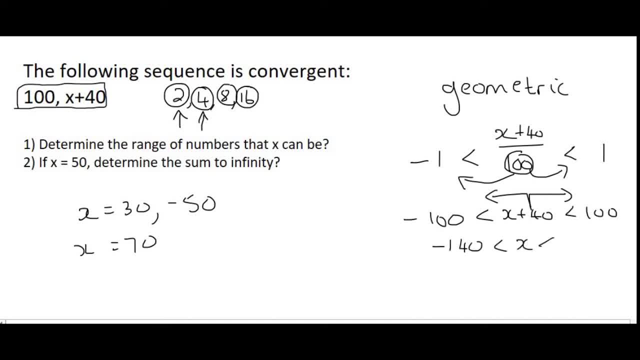 up with x being bigger than minus 140 and smaller than 60. So look what this says. It says that for the ratio to be between minus 1 and 1, x has to be any number in between minus 140 and 60.. 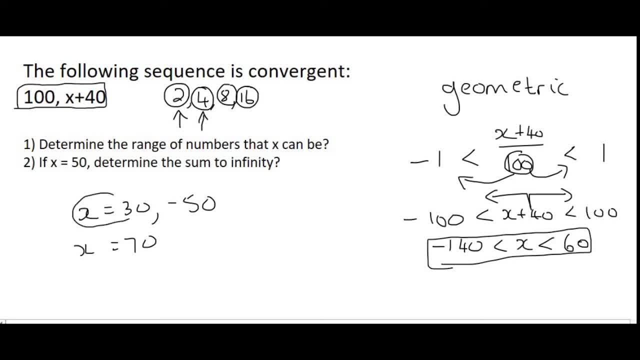 And that's what we found. We found that when x was 30, the ratio was less than 1 and bigger than minus 1.. And when x was a minus 50, it was also true. But as soon as x became 70, then the ratio 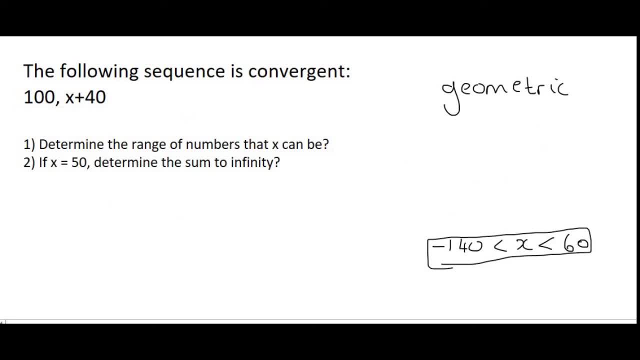 became more than 1.. And so, for number 1, determine the range of numbers that x can be. Here it is: x can be any number that is between minus 140 and 60.. Number 2 says, if x is 50, determine. 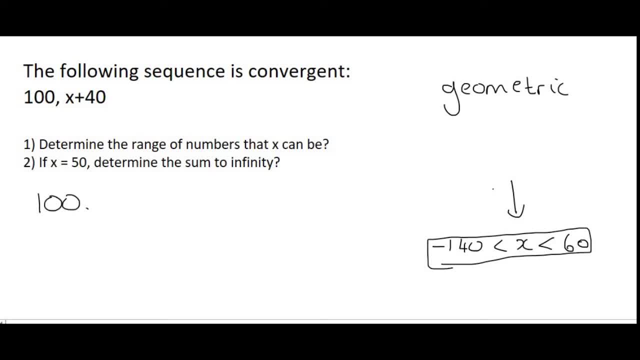 the sum to infinity. Well, if x is 50, then your first term is 100, and your second term would be 50 plus 40, which is 90. Now the sum to infinity formula can only be used on a convergent sequence. But we know that it's convergent because we just found the we, we found the x values that. 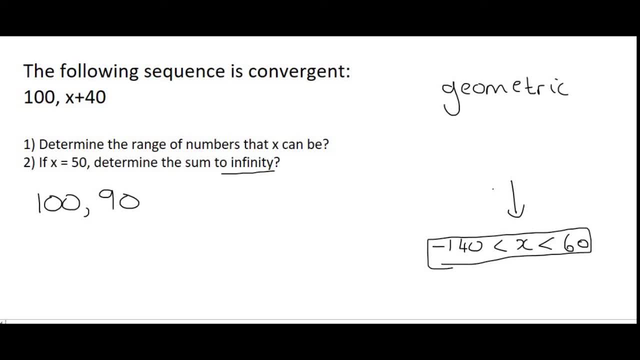 would make it convergent, And that's between minus 140 and 60. So if x is 50, which is in between those two numbers, then it's going to be convergent. So we are allowed to use the sum to infinity formula which we saw in the previous video. goes like that, And so a is just 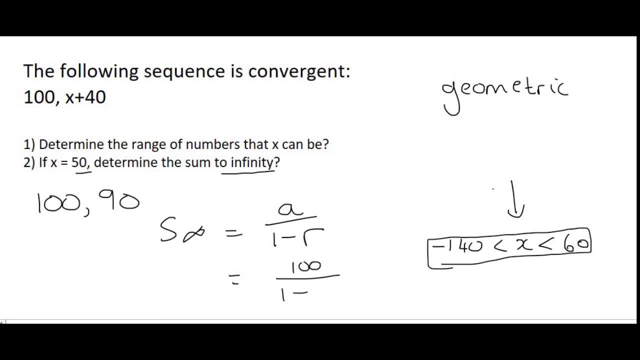 going to be term 1, which is 100 over 1 minus. Now r is your ratio. So the ratio here is going to be 90 over 100, which is 0,9, and that's going to give us a 1000.. So the sum to infinity is a.